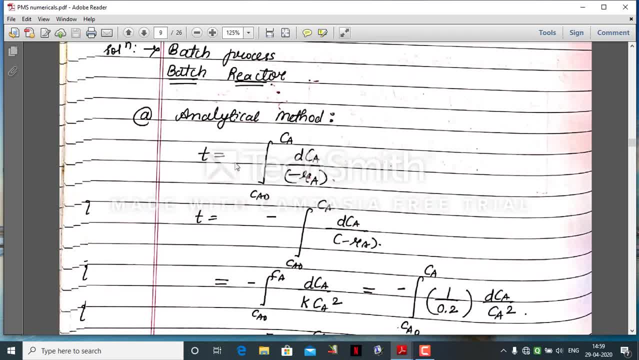 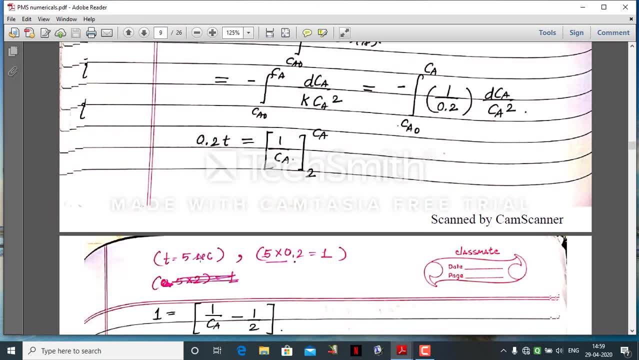 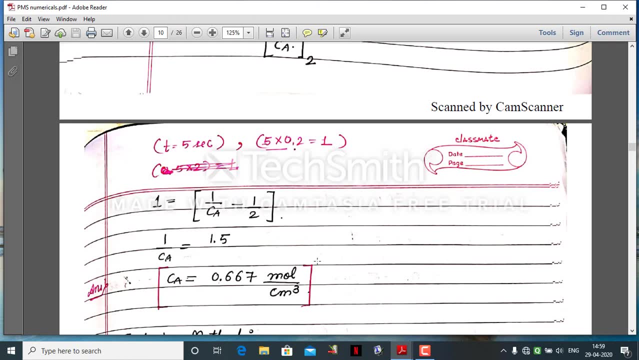 and we have. you can see, here we integrate this equation by putting the proper limits and by putting the value of t as a time. t is equal to 5 second. We have the concentration of a 0.667 moles per dm cube. Now, same problem we are, we will solve by using: 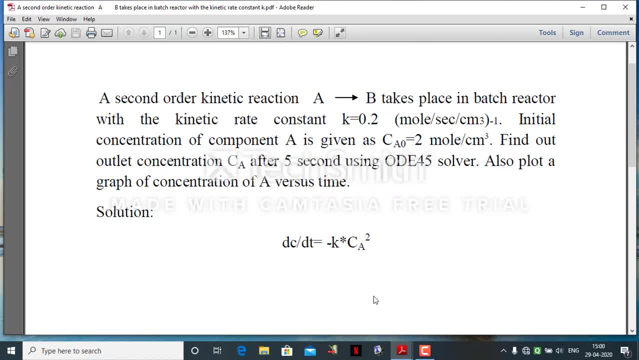 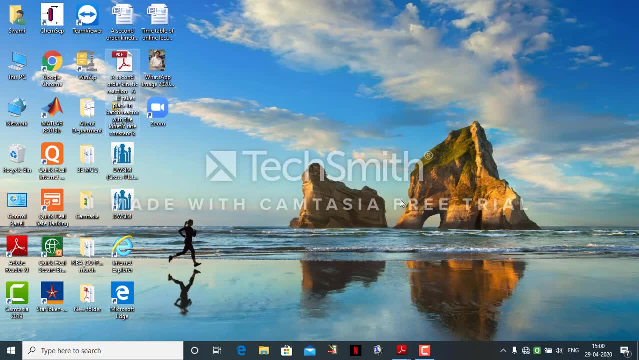 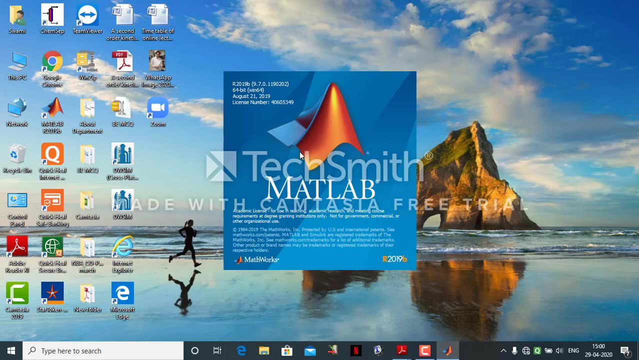 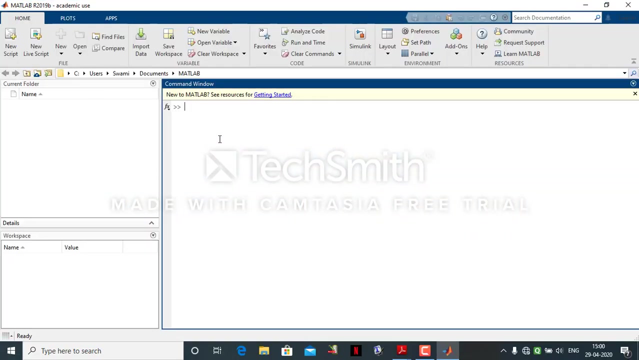 ODU solver in MATLAB. So for that we will open the MATLAB software by clicking on this icon. It will open and we will have these windows. So this is a command window, current current folder workspace. Now command window will execute the results and we are going to write our program in. 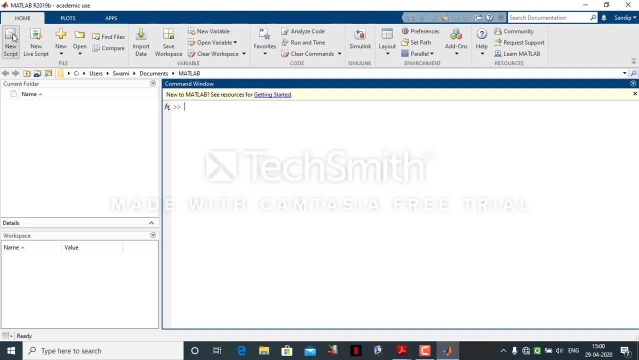 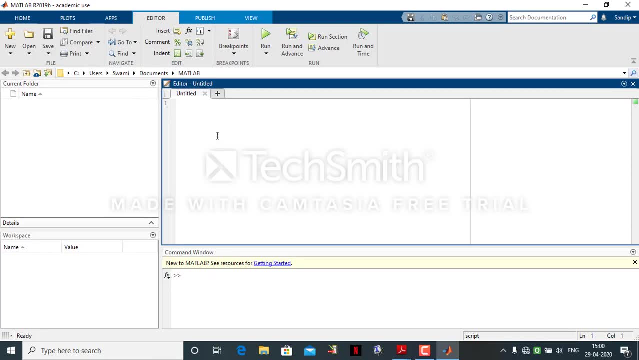 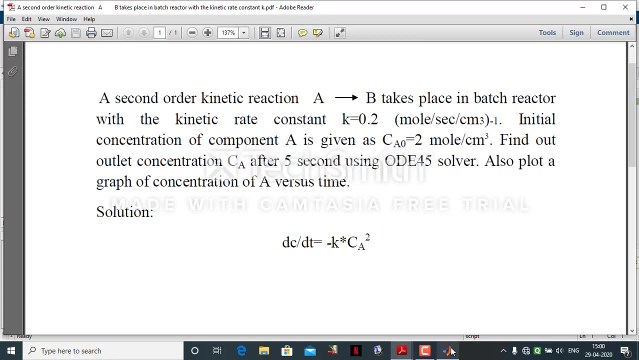 a script file. There are two different types of script file We are going to write our program in. one is a function file, or there is a script file or a data file. So we are going to write the equation or the function in function file and rest of the things in the editor file. So here 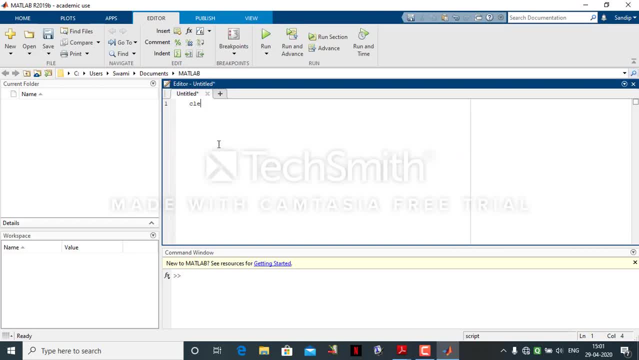 it will start from the command. that is clear, all close. all This can be used to remove the previous variables. we have assumed, Then, as we have to solve the ordinary differential equation, the best way to solve any softwares by using a simple command, that is zf1, that means help. So, similarly, as we have to solve that equation by, 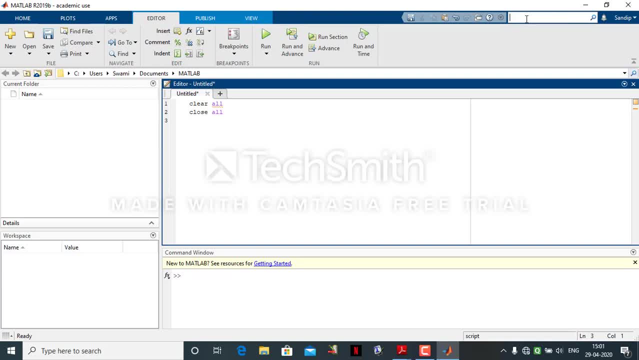 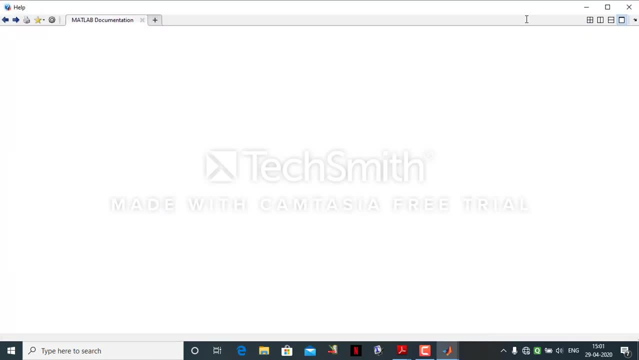 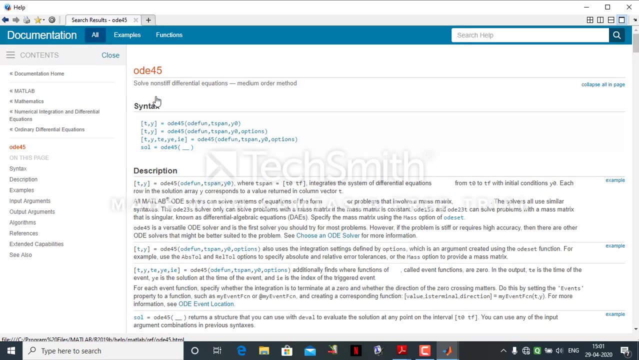 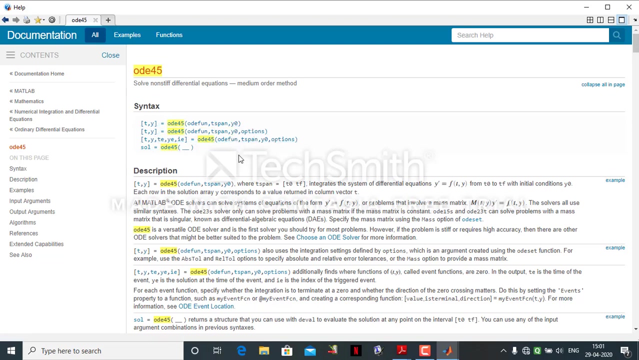 that is ordinary differential equation. we can take the help of this command, that is, ode45.. By putting on that there is a different helps we are obtained. So we will use ode45 command and the syntax is provided. Different syntax is provided here and we will use one of the syntax here. Now we will use this first. 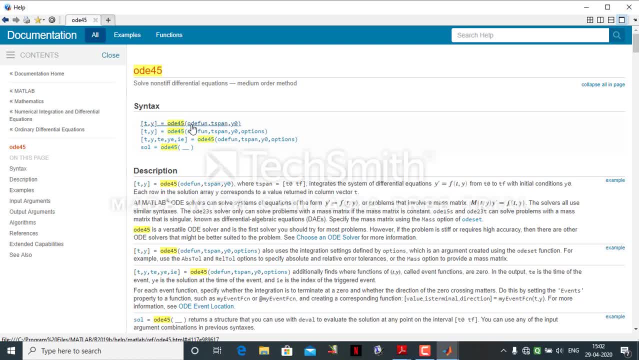 one that is t comma y, ode45 comma t comma s, t comma t span y0.. So ode45 is nothing but the a function file, ode45 is a solver, t span is a time and y zero is nothing but the concentration, initial concentration of the dependent variable. Now we will see how to solve by using MATLAB. 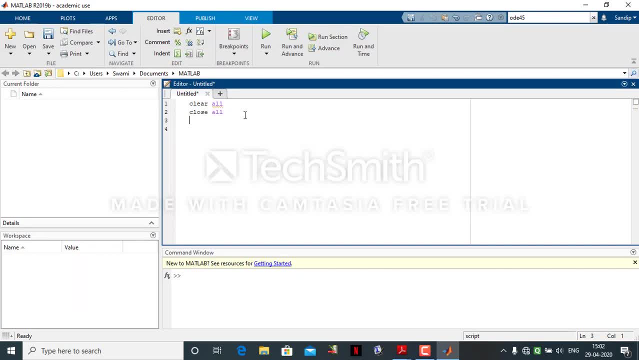 So here we will use that command, that is tc. tc equals t to ODE45. so here, as we type ODE45, it helps us how to write that syntax. so here we have to write ODE function file, so we will give the name, that is batch reactor. fun fun means. 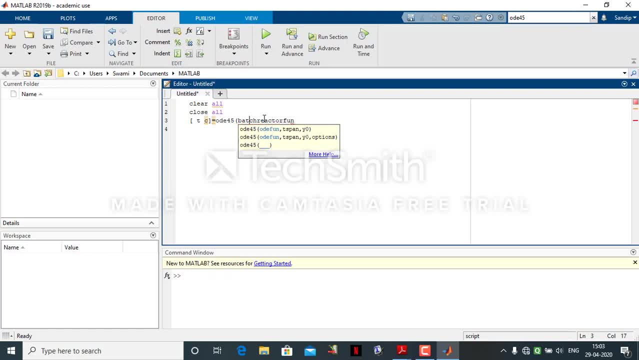 function file. so before that we have to write here semicolon, single inverted comma. then we have to write TSPAN, then initial concentration, that is C0. now, before writing this here, the syntax we have to write, we have to provide all these TSPAN and then we have to write. 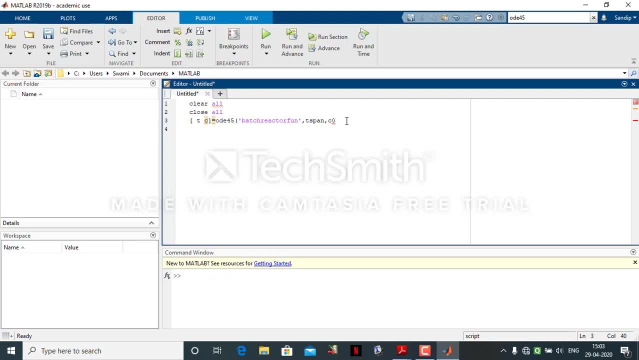 TSPAN and C0, that is initial concentration or initial values. so before that we give that values, that is, TSPAN or C0, we will give first of all C0. C0 equals to, that is 2, which is already provided. then we will write TSPAN. 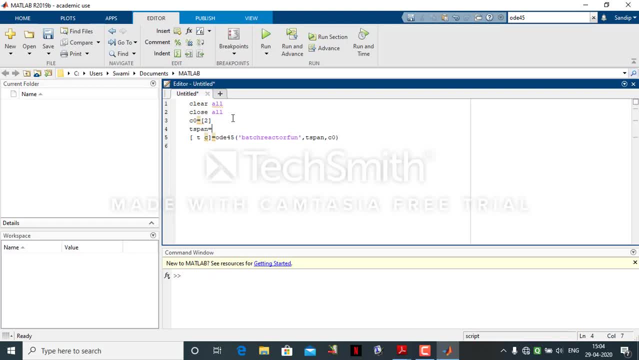 that is 0 as to, will take a step size of 0.5, and we have to find out the concentration for 5 second. so that's why 5, this is the syntax. now we will have to plot the graph also, so we will write for it. for that, plotting the graph, that is the command. PLOT, that is plot. 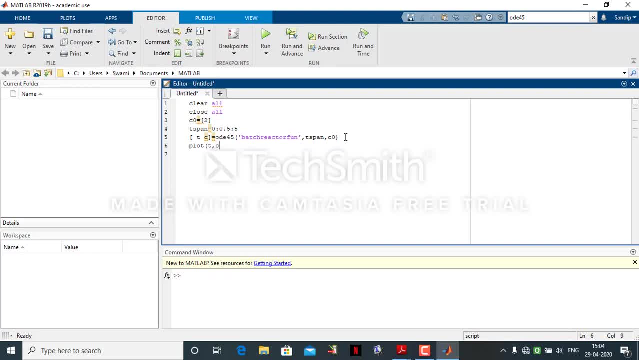 of TSPAN. then we will also give the title to that plot, title: concentration versus time. then we will give x level. that is a name for x-axis. on x-axis it is time time in second. on y-axis it is y level, we have concentration. 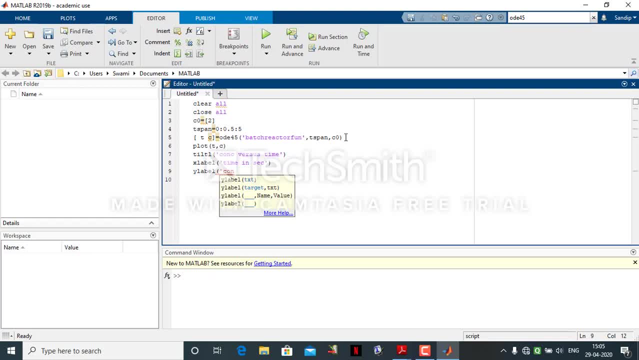 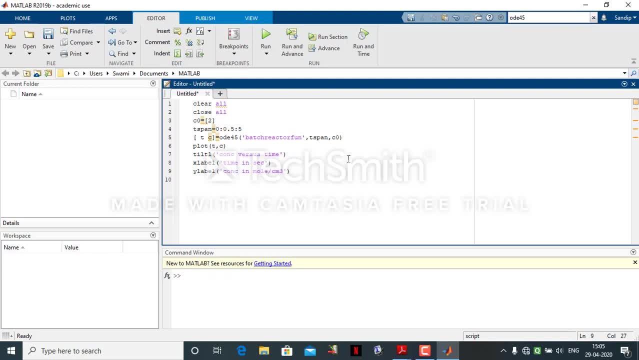 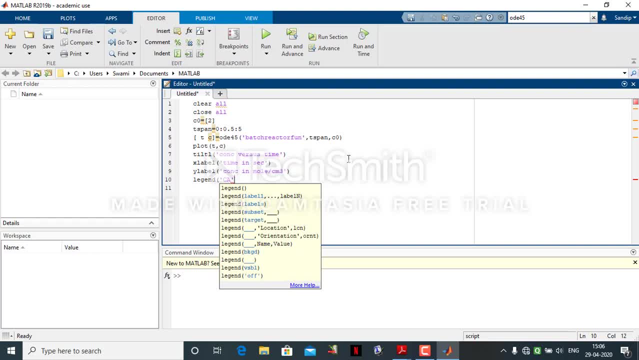 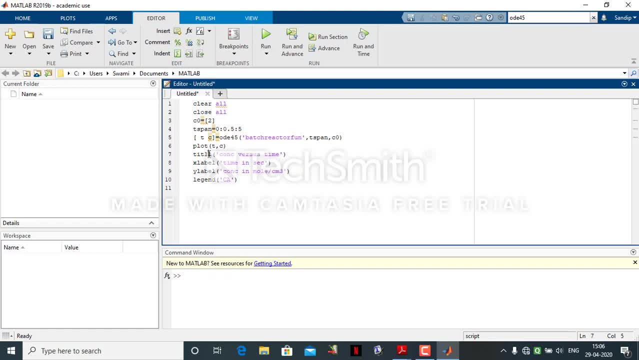 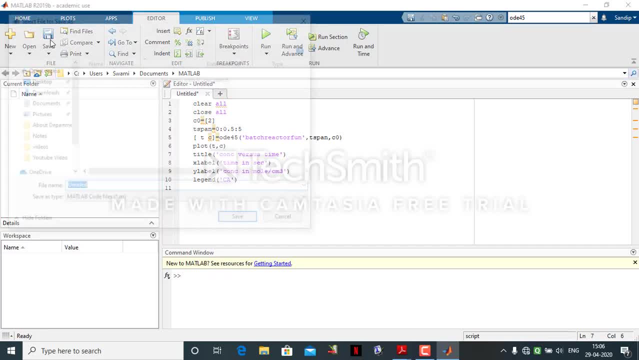 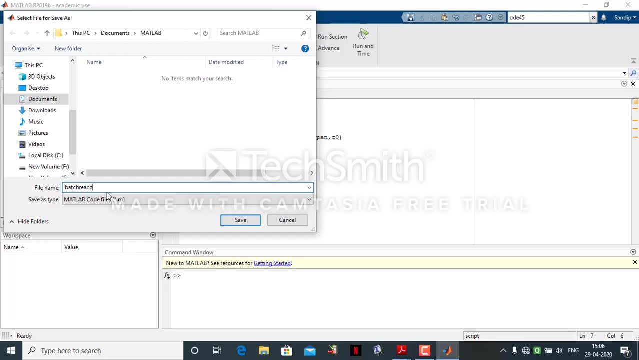 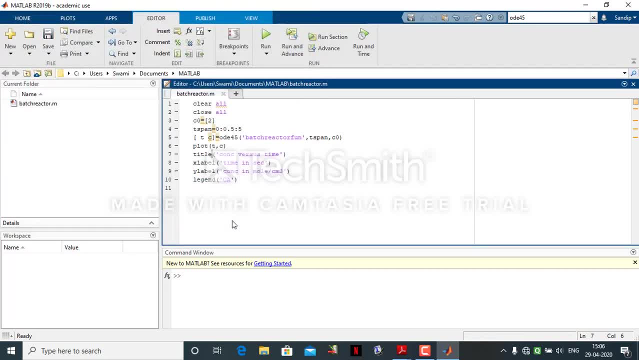 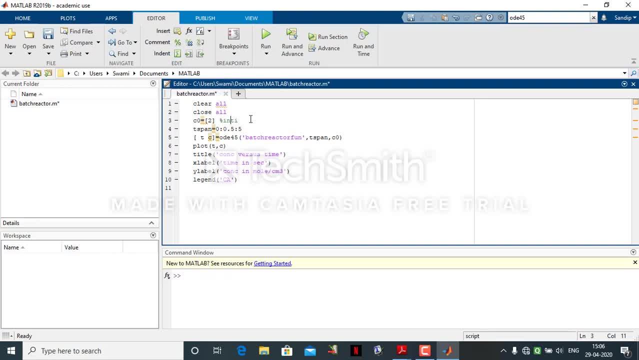 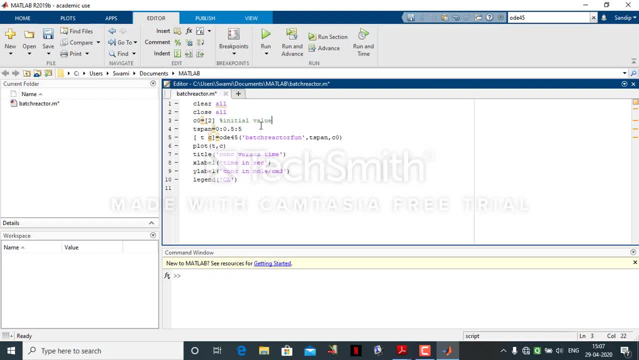 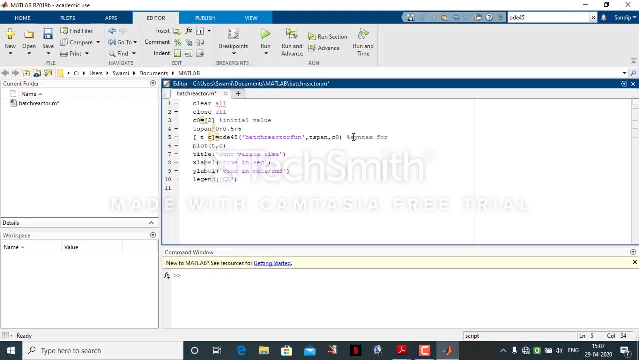 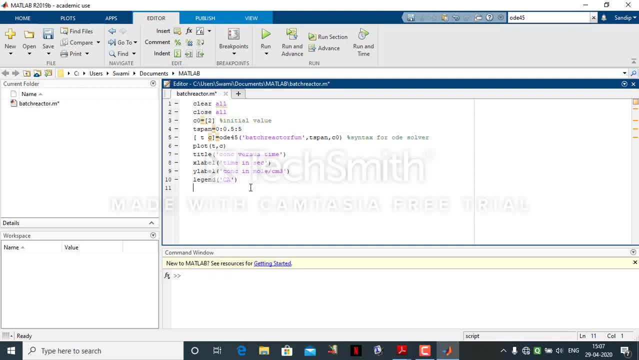 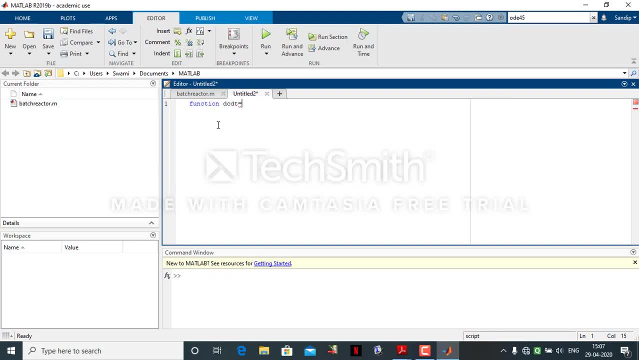 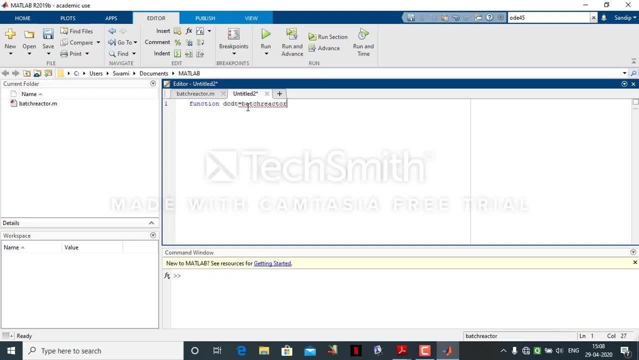 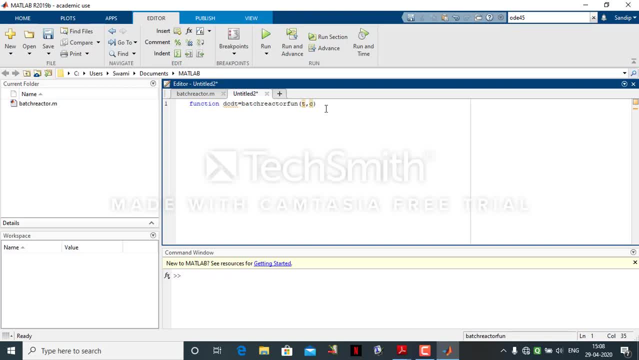 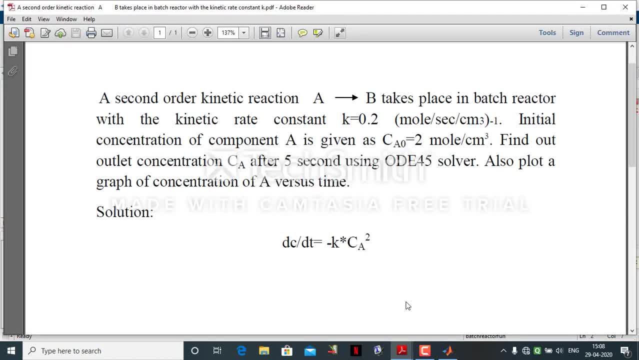 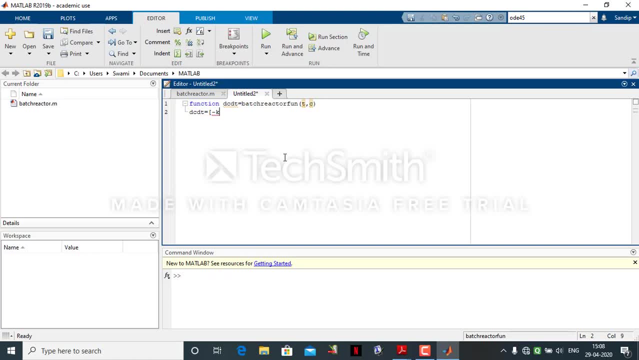 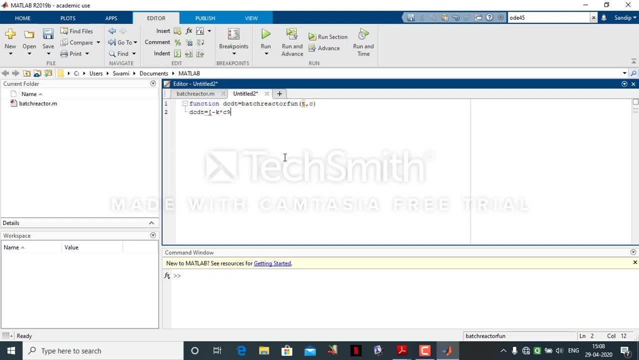 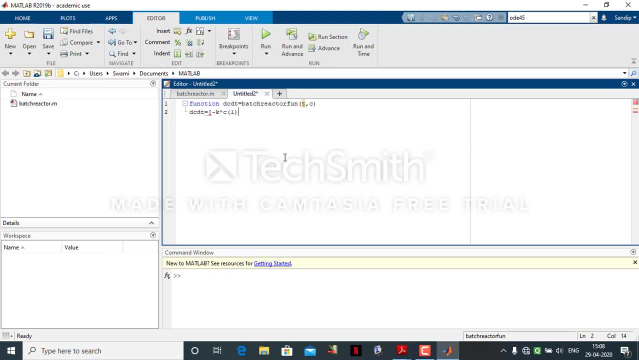 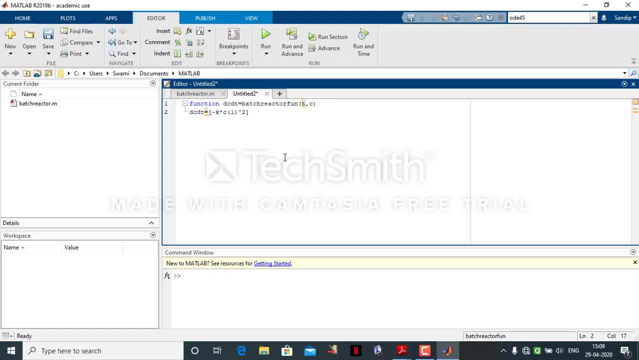 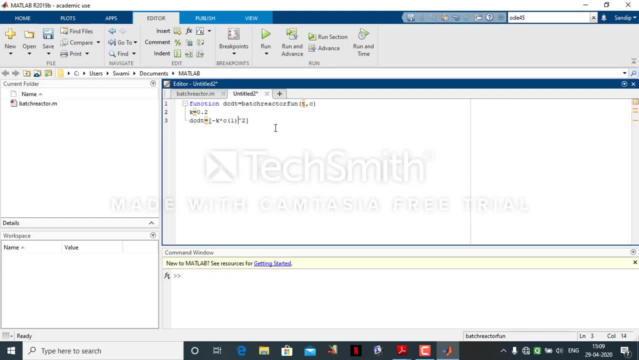 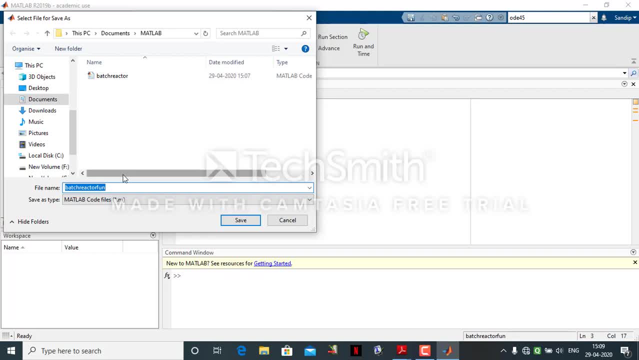 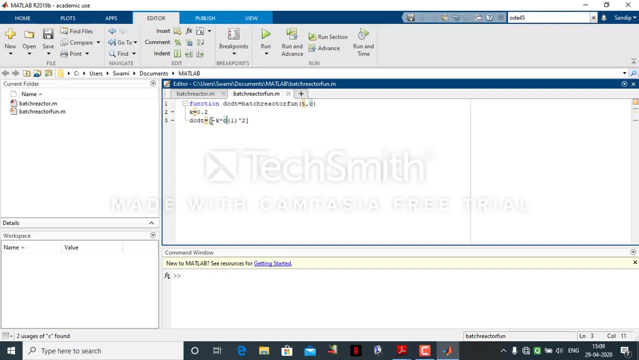 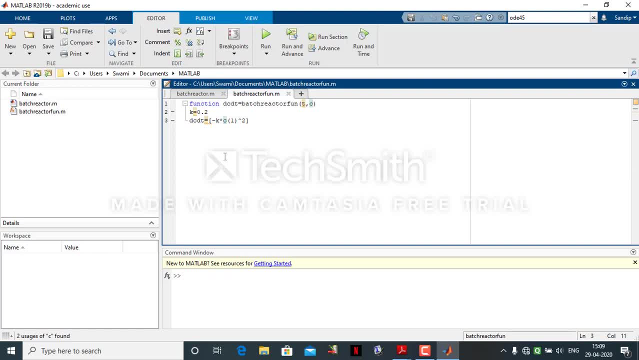 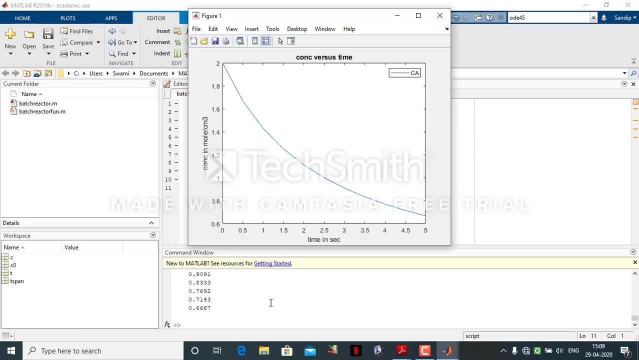 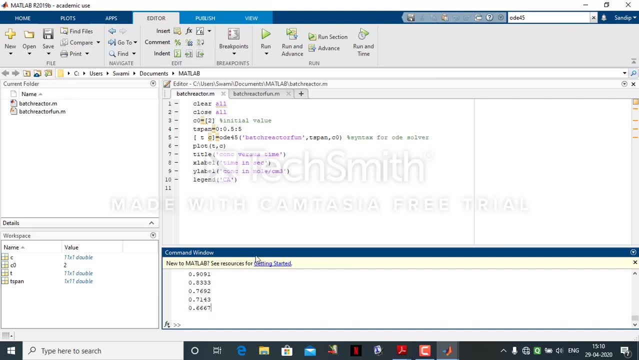 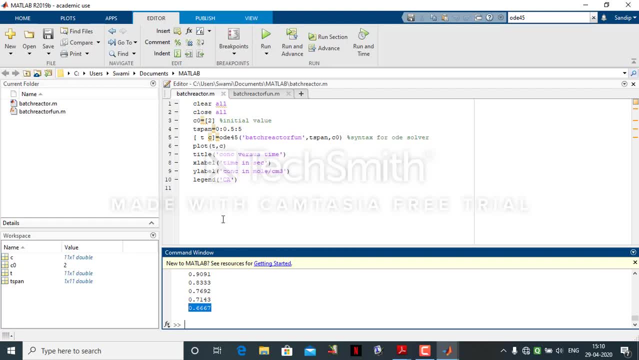 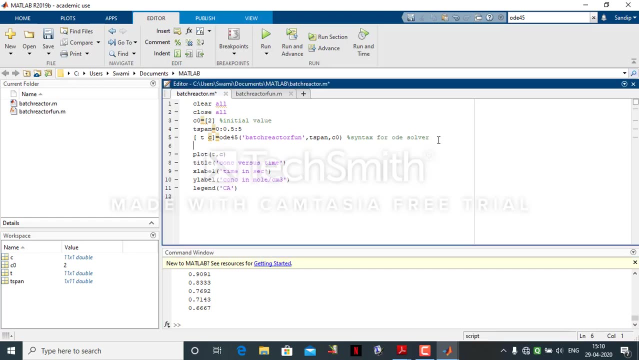 a after five second. so this is the value. now we can get that value. how much? uh, how we can identify this? uh, this is the function or this is the value, that is: 0.667 is the concentration after five second, so that here we can also add one line here that is: results. 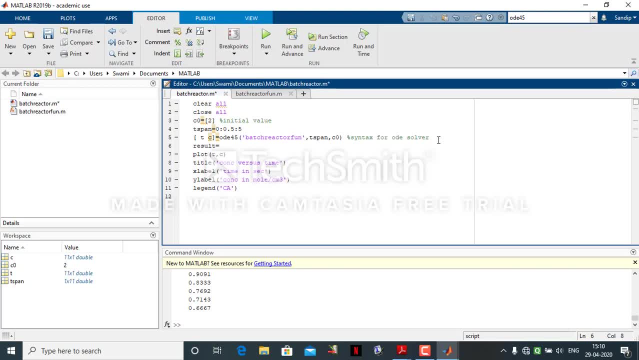 is equal to, and here we can put time and c. so this vector and after whatever we make a change, we have to save it, and after saving it, then we can, then then only that change will uh execute in the function. then again we can run this command. we will have. 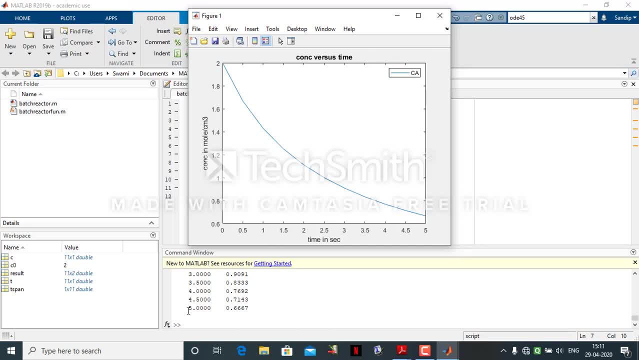 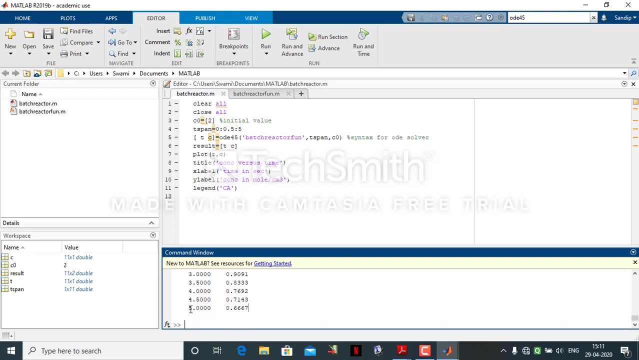 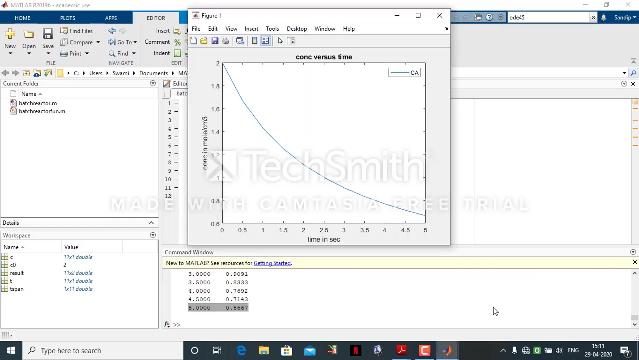 see, here we got the plot and also we have this uh equation that is this: results. that means this: this is a time vector and this is a concentration vector. so after five second we have this value and also we have this figure function. from this figure function we can see here the name of the 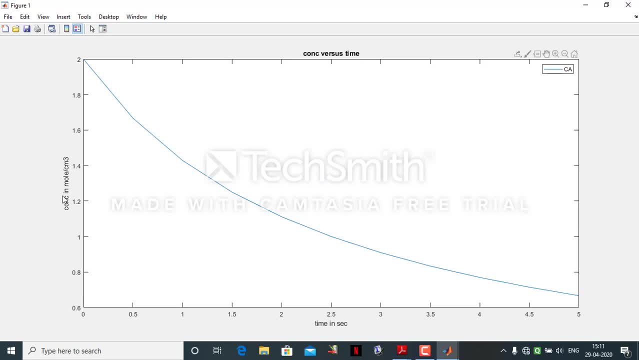 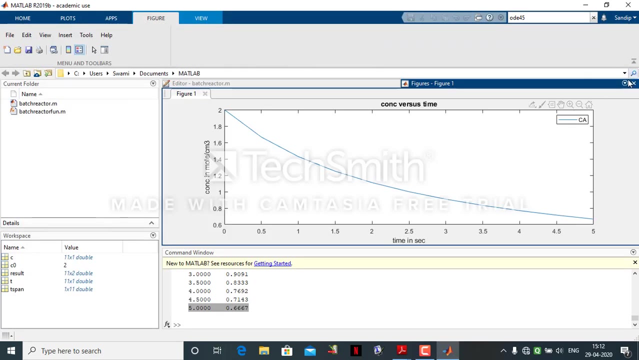 this title of this graph is concentration versus time. uh, on y-axis, concentration and concentration in volts per cm cube. x-axis is also given and this legend for this is c. in this way, we can uh have this uh graph also graph value. now, uh, as we can uh this, uh, as we change this con.